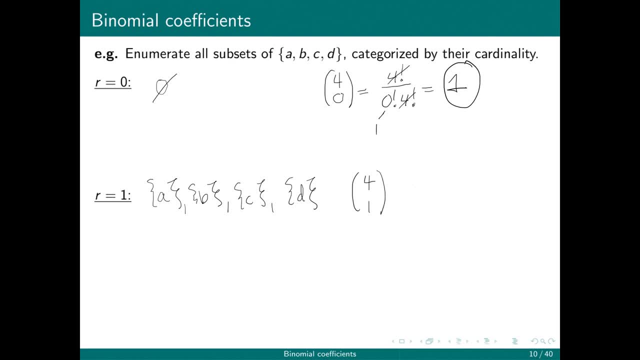 those. so 4, choose. 1 had better be equal to 4 or factorial divided by 1 factorial, because 1 is R and then n minus R is 3 factorial. remember we can write 4 factorial as 4 times 3 factorial 1. 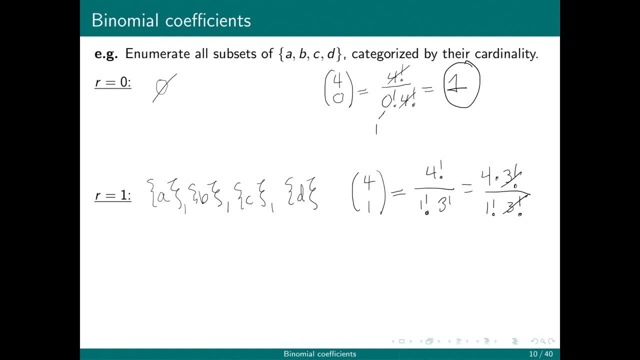 factorial is just 1, we can cancel the 3 factorials and, sure enough, we've just got 4. all right, you? this is a little harder to write down, all the two elements, subsets. I'm going to be systematic about it, so I'll do all my a's: a, B, a, C, a D. actually, this is just. 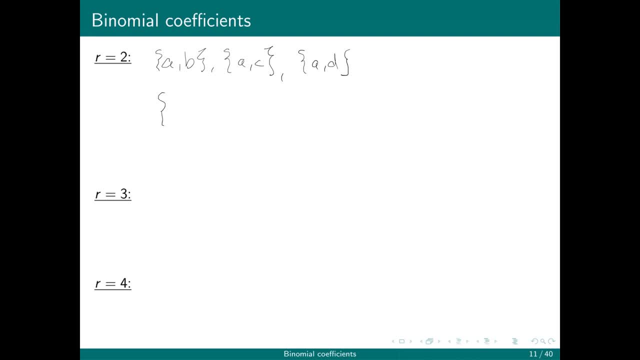 the example we did in the last video. right, all the unordered samples of size 2. that needs to be a B and then that's CD B. all right, I think you already knew there's six of those from that example last time, so we're gonna have four. choose two is four, factorial over two. 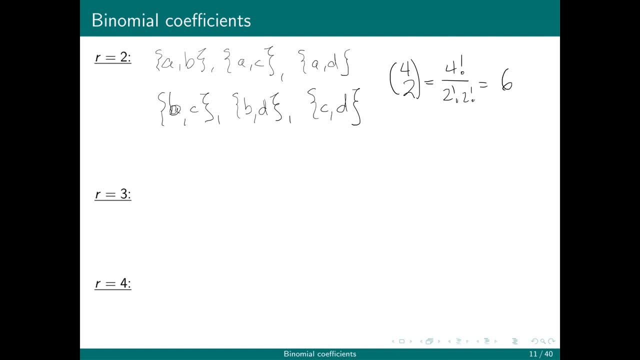 factorial 2: factorial, which we already new was six, all right. next up, we're gonna have a B C a, B D, A C D and B C D 4. choose 3 is 4 factorial over 3. factorial 1: factorial, which is equal to 4, and so I want you to notice a couple of things, notice. 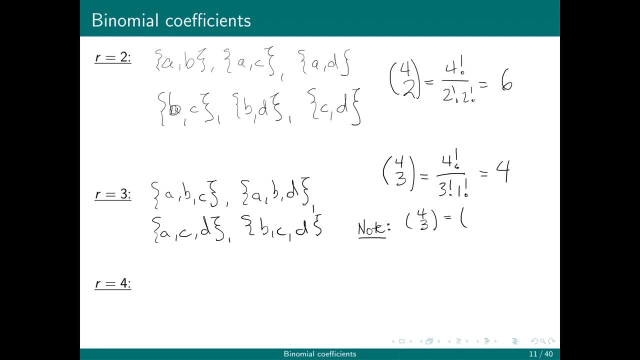 that 4 choose 3 is just 4 choose 1 and that's clear from the algebra right when we write this number down. 4 choose 1 is 4 factorial over 1 factorial, 3 factorial. so the only difference is the order of the numbers on the bottom of the fraction, and of course that doesn't matter, because I'm 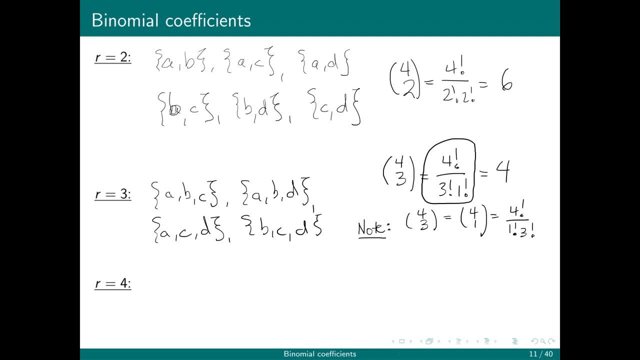 multiplying those numbers together. so algebraically it's clear that 4 choose 3 and 4 choose 1 are the same number. another way we can think about the relationship between 4 choose 3 and 4 choose 1 is that when I'm counting 3, 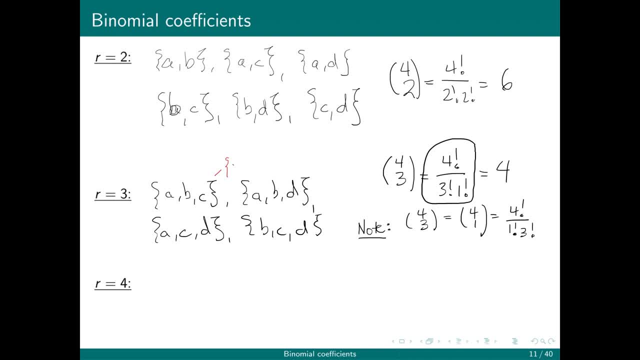 element subsets, I'm having to leave behind another element. so, for example, the set ABC has its complementary subset, as the set containing the element D, ABD has as its complement the element C. ACD leaves behind B and BCD leaves behind a. so for each one of the three element subsets there is exactly one one element subset that I'm 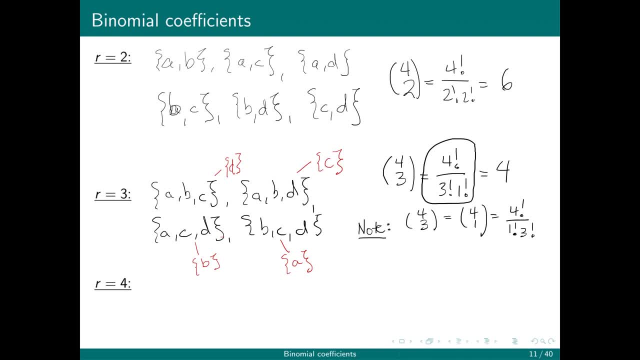 leaving behind and vice versa. so there better be the same number of those. we'll talk about that in a little more detail in just a minute. and then there's only one. wouldn't be a video without that. there's only one four element subset. having some trouble with this today, there we go. 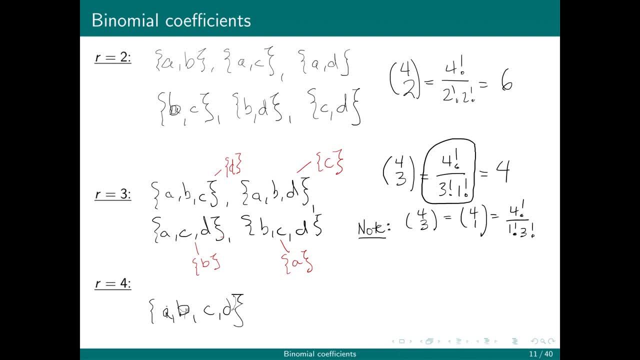 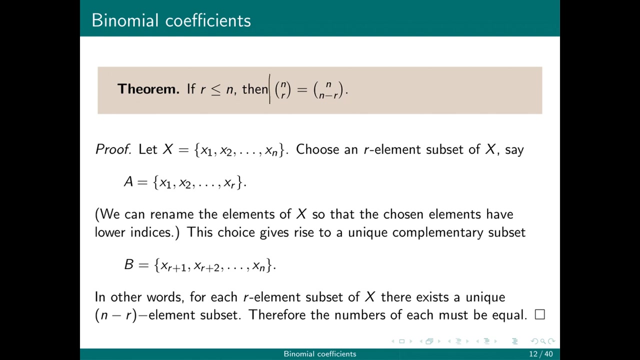 of course, when I take all the elements, I'm leaving behind nothing. so there's exactly as many four element subsets as there are empty subsets. so here's the theorem for that in choose R is always equal to N, choose N minus R. and here's a proof. it is basically exactly the example that 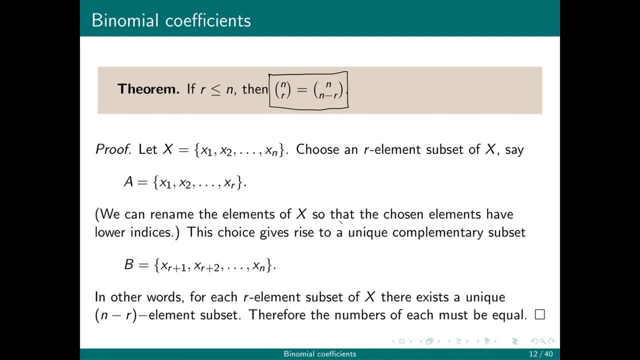 I just laid out, just kind of made general: we're gonna let X equal the set X, 1, X, 2, dot, dot, dot X in and I'm gonna choose an R element, subset of X and I'm gonna call it a, and what I'm gonna do is I'm 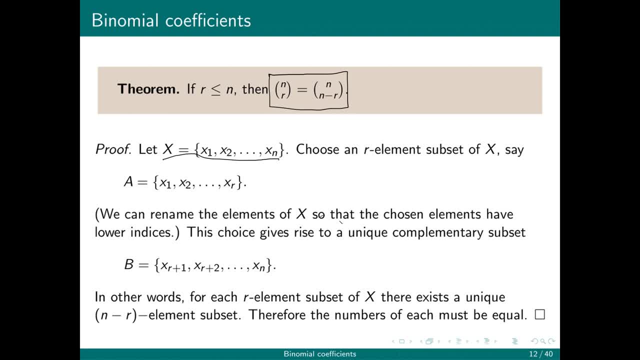 going to rename the elements of X. I can do this whenever I want. doesn't matter what the elements of a set are called. all that matters is how many of them there are. so instead of calling the elements of X whatever they were, I'm going to rename them. so the first R elements are: 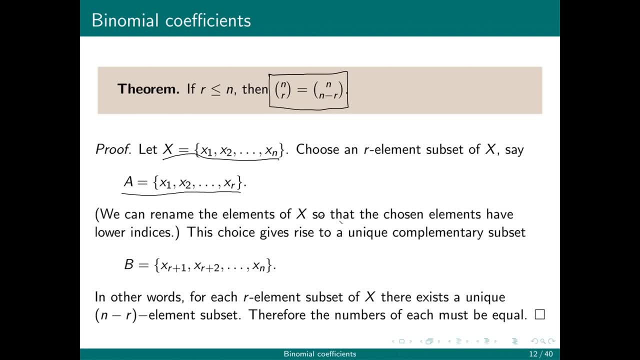 in the subset that I choose all right. well, if I choose X 1 through X R, then that means I'm leaving behind X R plus 1, X R plus 2, dot dot, dot X in, all right. so this is a R element subset. this is a. 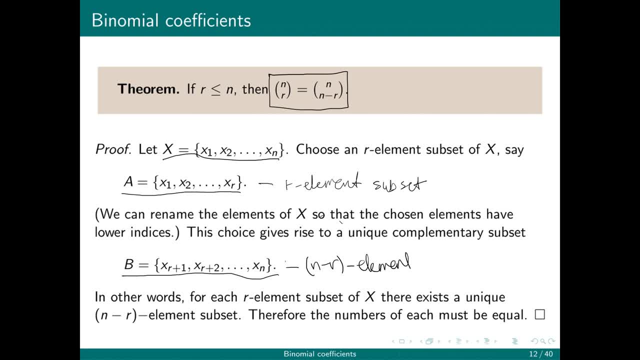 N minus R element subset and there's a perfect correspondence between these: for every a there's a B, so there have to be exactly the same number of them and therefore N choose R is equal to N choose N minus R. 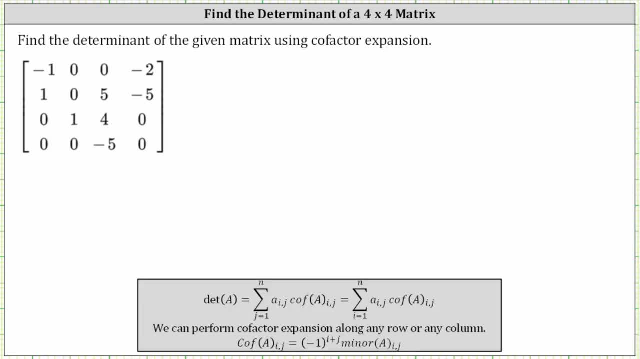 We're asked to find the determinant of the given matrix using the cofactor expansion method. To find a determinant using the cofactor expansion method, we can select any row or any column and we multiply each element in the row or column by the corresponding cofactor. 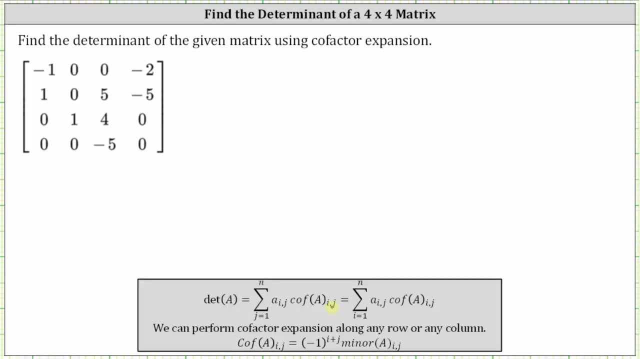 and then we find the sum of all the products. So it is worthwhile to analyze the matrix and select the row or column that contains the most zeros, because that will reduce the amount of work to find the determinant. So, analyzing the matrix, notice: row four contains three zero entries. 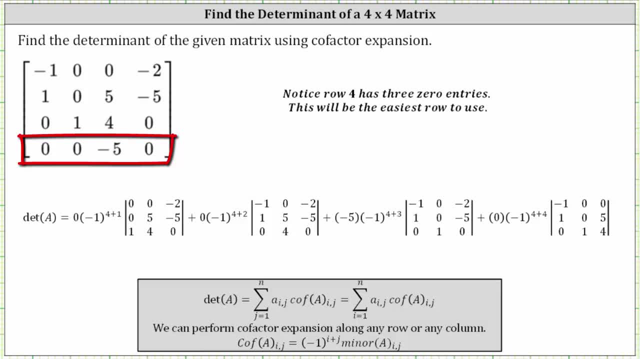 and therefore it'll be less work to use the cofactor expansion method along row four. We begin with the first element in row four, which is in row four, column one. So we begin with zero and then, because the element is in row four, column one, 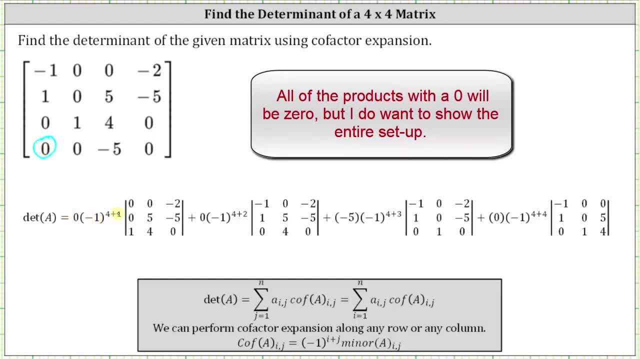 we multiply by negative one, raise the power of four plus one. Next, we eliminate row four and column one from the matrix and multiply by the determinant of the remaining matrix. Notice how we have a three by three matrix where the first row is zero, zero, negative two. 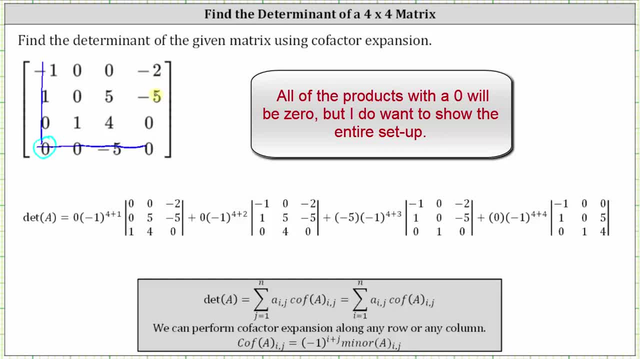 the second row is zero five negative five. the third row is one four, zero. So we have the three by three determinant of this matrix shown here. So here we have a sub four comma, one times the corresponding cofactor. And now you move along to the next element in row four. 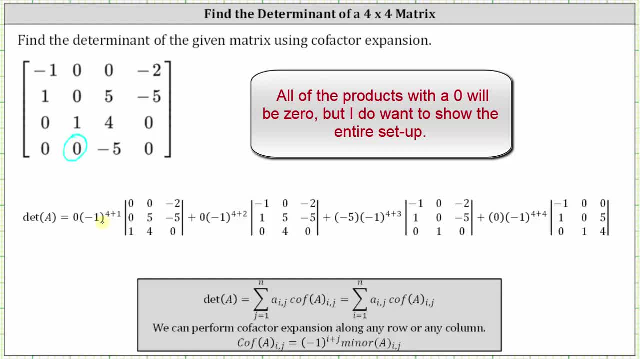 So we have plus. next element is zero, and this element is in row four, column two, And therefore we multiply by negative one, raise the power of four plus two, And then we multiply by the determinant of the matrix formed by eliminating row four and column two.